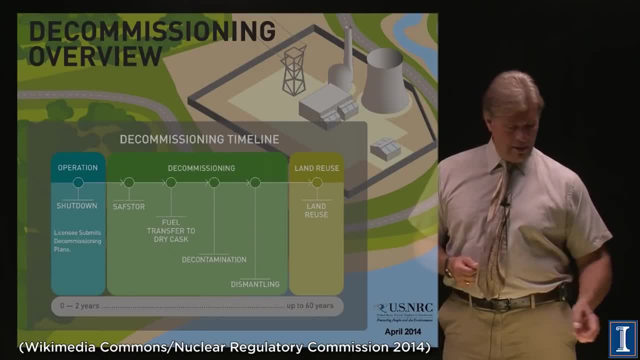 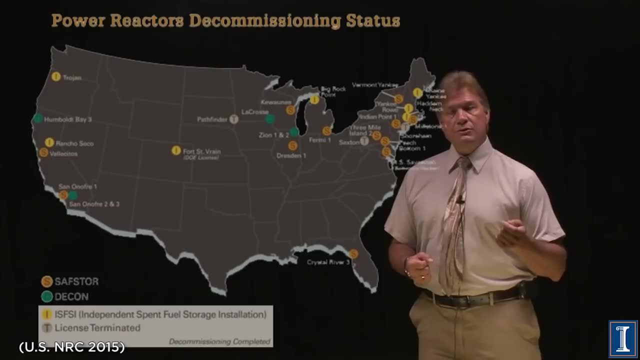 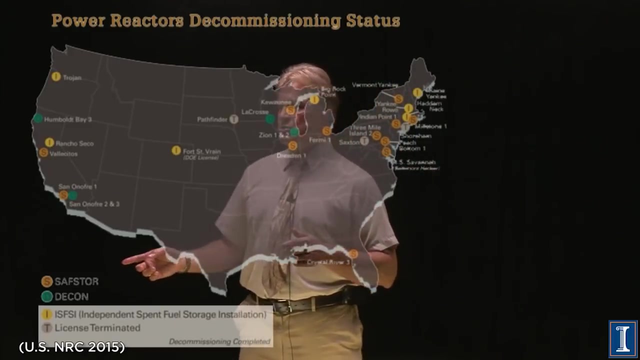 On it you had to remove. Well, this process has actually happened in the US at a number of locations and this means we understand the economic implication. You can see that there's some acronyms here. Safe store is where they basically take the hottest things. 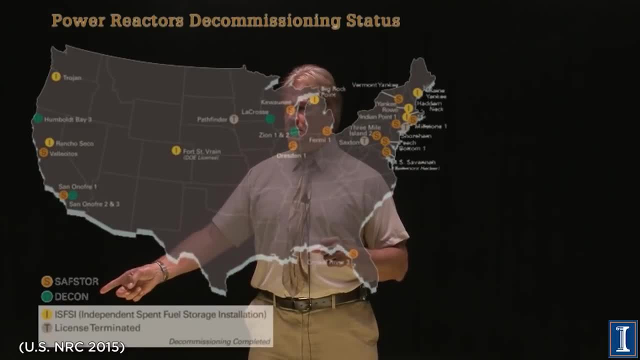 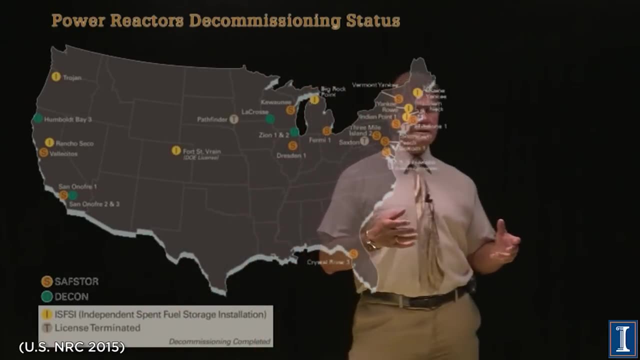 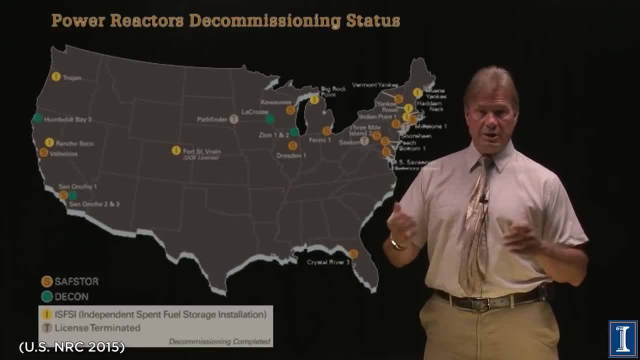 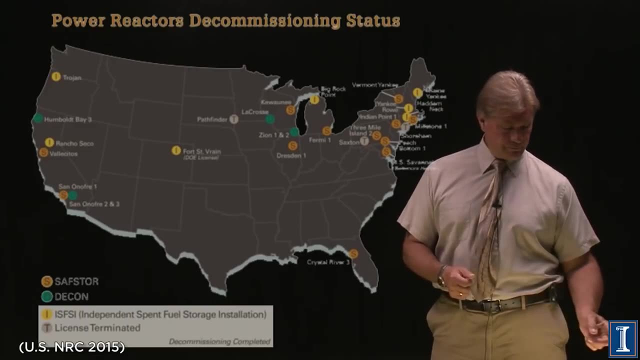 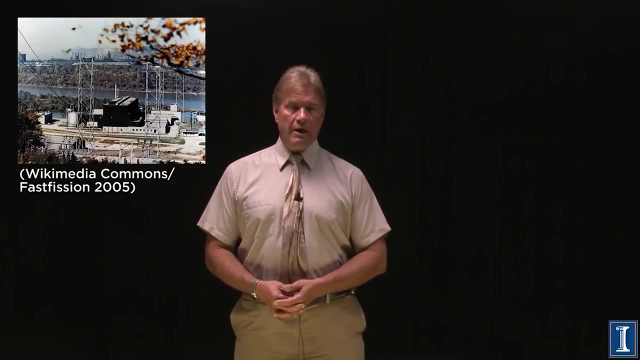 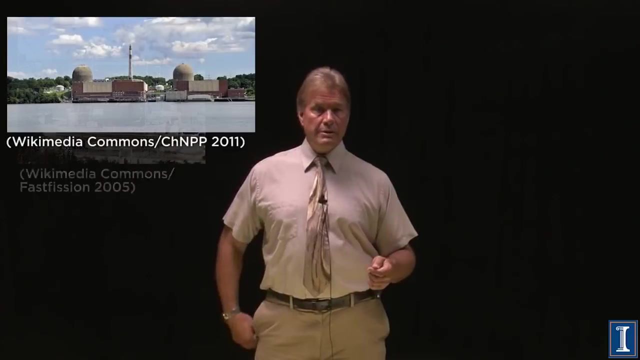 And you can't go back and see the codes that you've put up there, And it's not really a good time to sit there and be thinking: you know, I don't know what's going on here. No, I don't. 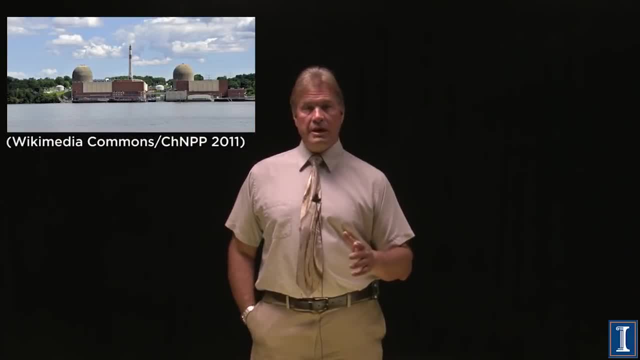 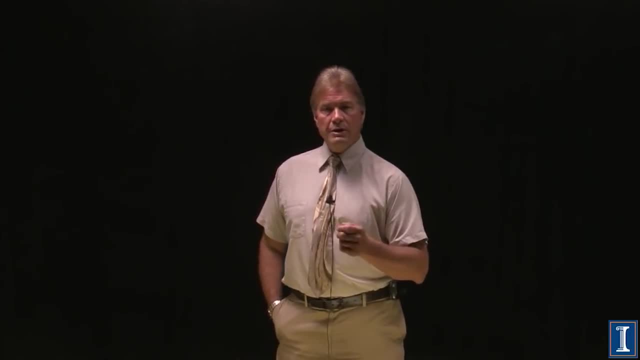 No, No, No, No, No commercial reactor. It ended its life in 72, and it's been fully decommissioned. There's a large list that have, and so the costs are well known And fortunately early on there. was a law in Congress that said: out of every kilowatt hour of electricity you sell, you need to save a little bit of that profit- Something on the order of a tenth of one cent from every sale that goes into a decommissioning fund, so that at the end of your reactor's life. there is a pot of money there to be able to take it apart And the utilities have done that and they've done it quite well. The costs today are about 300 to 400 million dollars to take apart a nuclear reactor and that money is there. That money is monitored. 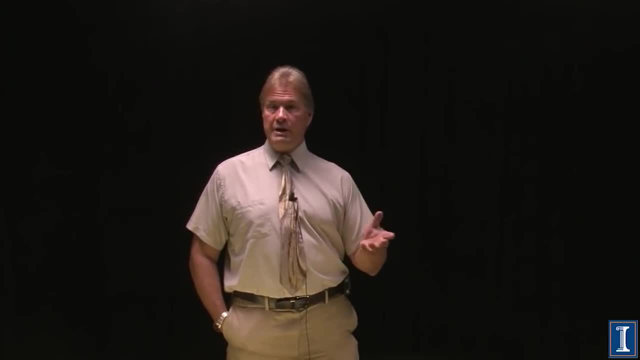 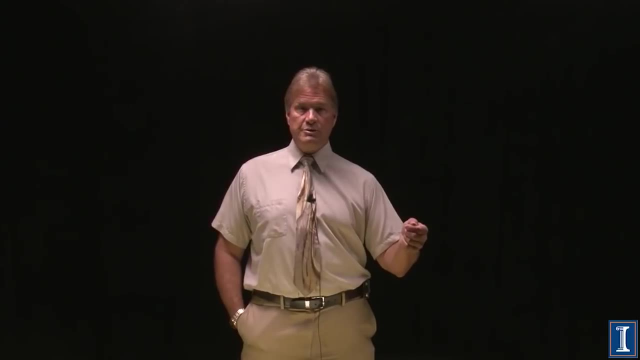 by the Nuclear Regulatory Commission to make sure that there's going to be enough. Sometimes there's adjustments, Subtitles, by the Amaraorg community made in terms of the amount a particular utility has to charge their customers, or maybe even decrease that amount because they want to make sure that this money is there. 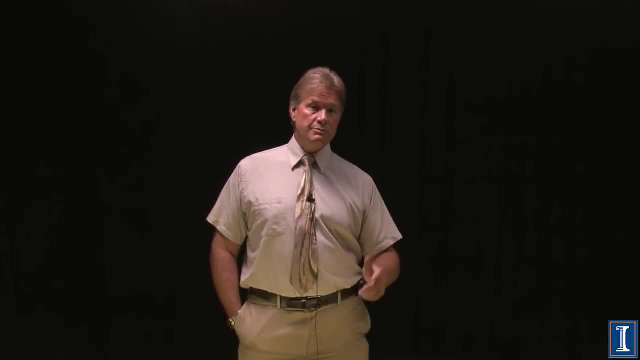 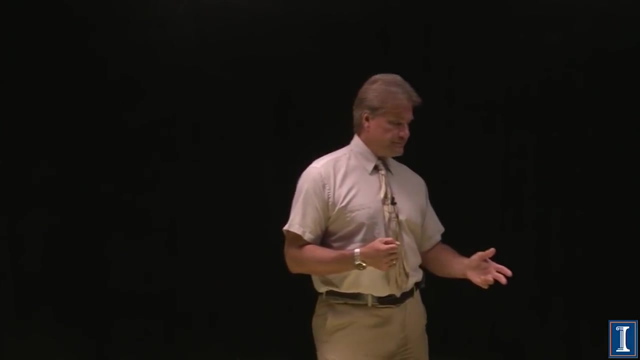 and earmarked for only that purpose, And the system has worked quite well. In addition to just talking about it, I have some personal experience in decommissioning. You see, at the University of Illinois we had a research reactor And the reactor was. 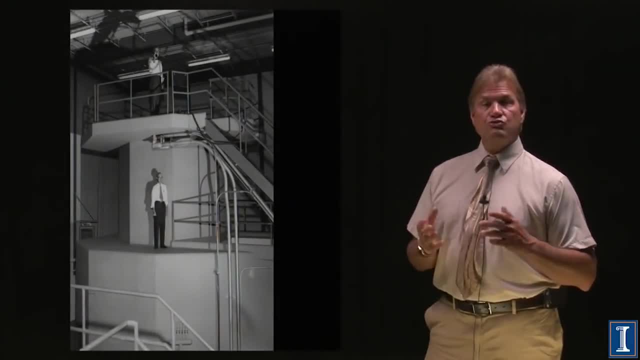 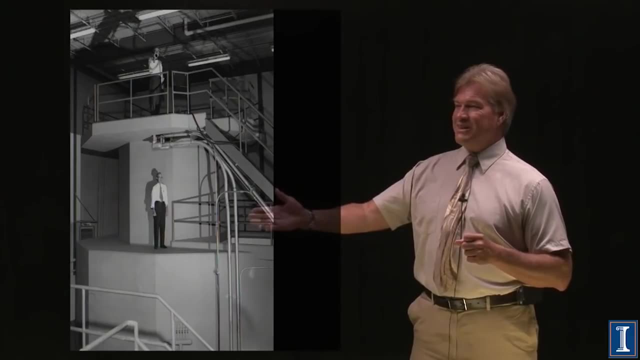 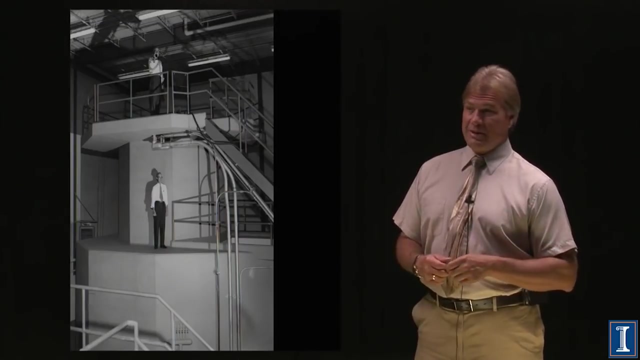 the type made by GE called the TRIGA, Training, Research, Education, General Atomics Reactor, And it was started in 1960. And this is the TRIGA reactor at Illinois. Well, 1960 was quite some time ago And the reactor had a wonderful, very useful lifetime, not just. 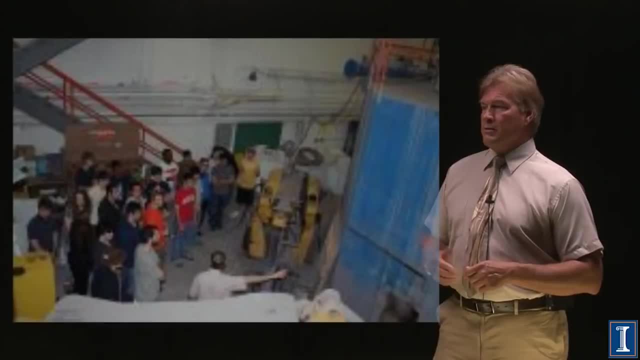 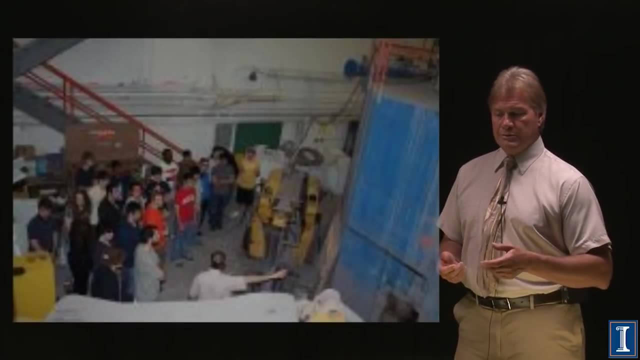 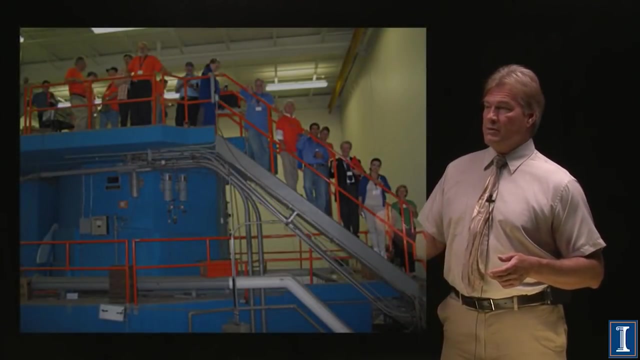 for research, but also for education. Lots of tours would go to the reactor. I remember running a lab class there to use the neutrons that were coming out. The reactor is a fairly impressive building. You've got people on it. The reactor core is down below the central. 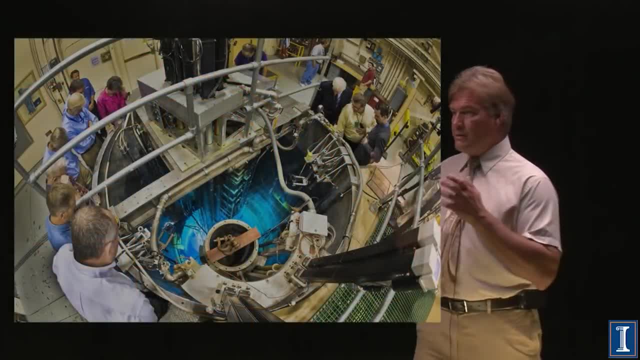 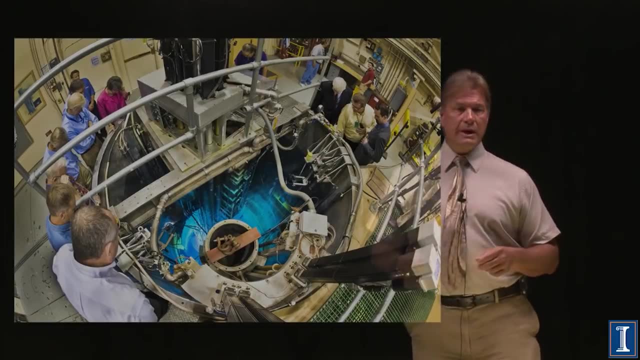 part. In fact, if you look down here, you're looking into the water And the core is at the very bottom And the water is very good shielding. So all of this took place, But 1960 to about the year 2000,. that's 40 years. That was the 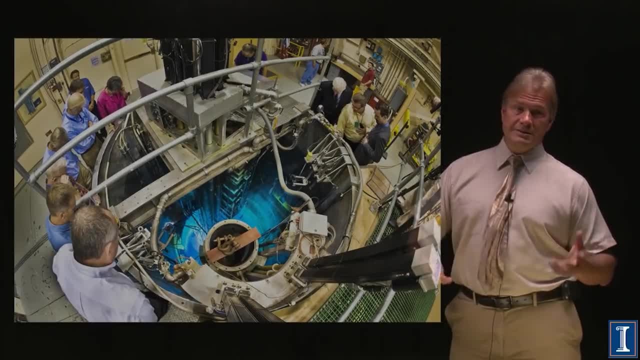 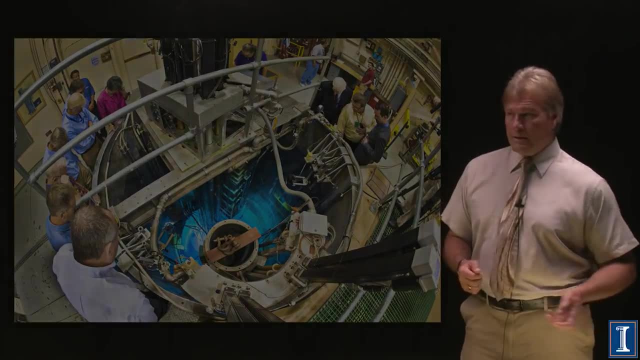 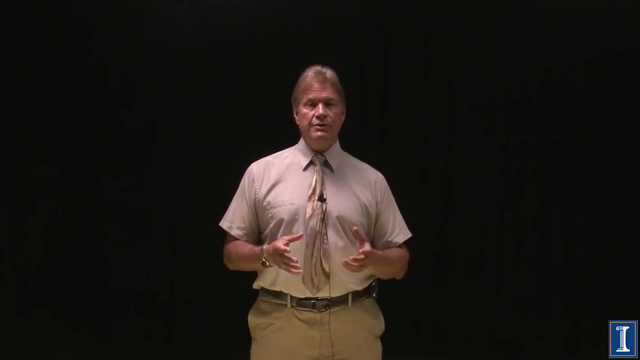 first time we had a reactor license. Technology is 1960s technology. Maybe there's some things you could do, but the decision was made to decommission And in this decision to decommission they actually had a deal back from the 1960s with the federal government that they would. 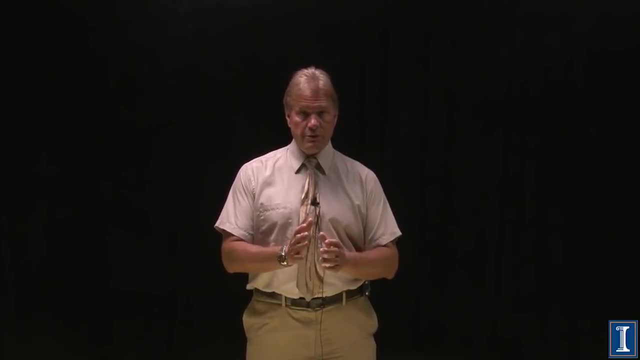 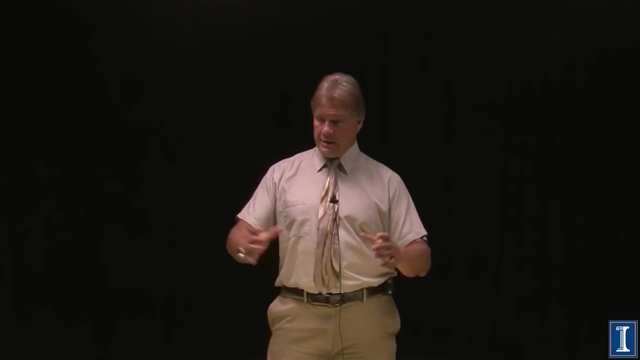 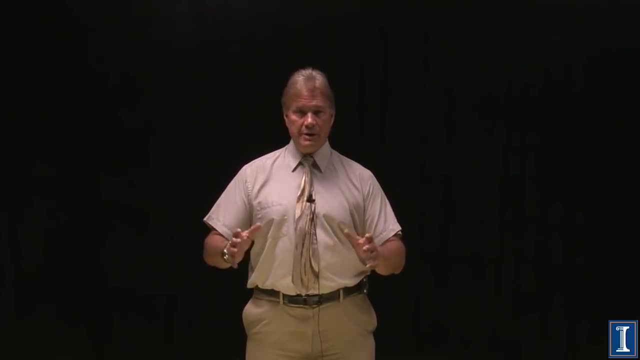 take the spent fuel, And that's excellent because the spent fuel, the stuff inside those fuel rods, is the high-level waste. So that's going. Now we have a reactor vessel inside those massive blue pieces of concrete. that is radioactive, And some of the concrete at least. 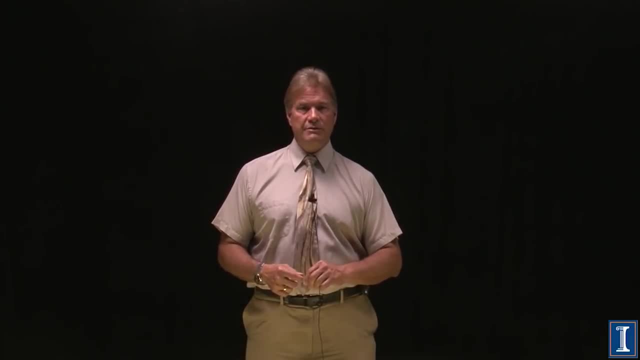 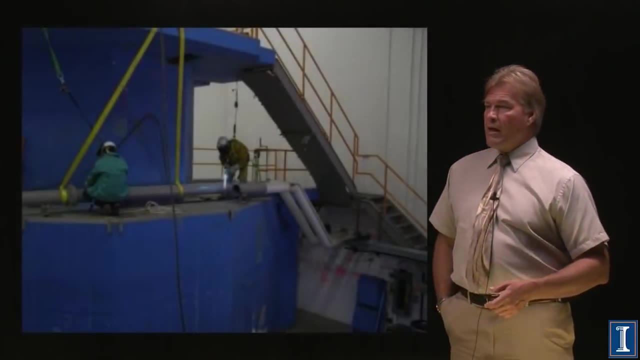 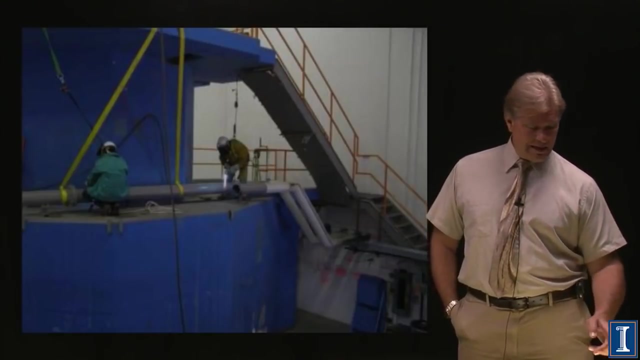 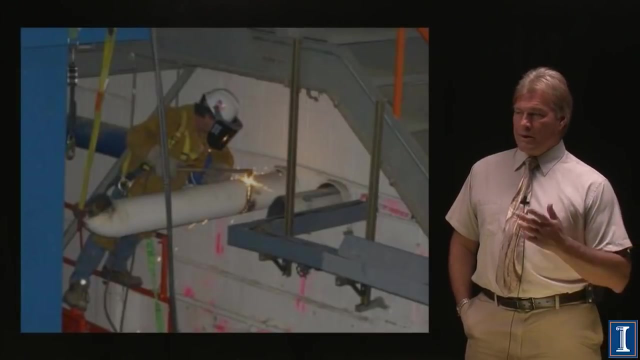 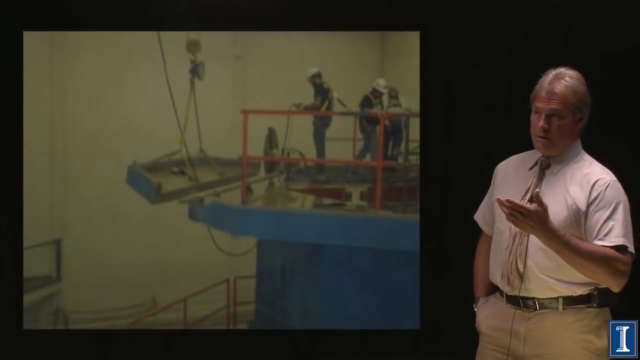 the stuff nearest by may be slightly radioactive. You've got to take it apart. So we did: Certified work crew monitored everything else, Start going in and basically cut things apart. You have people cutting off pipes, Sawing off all the things that go into the building, Even the pieces of concrete. How do you? 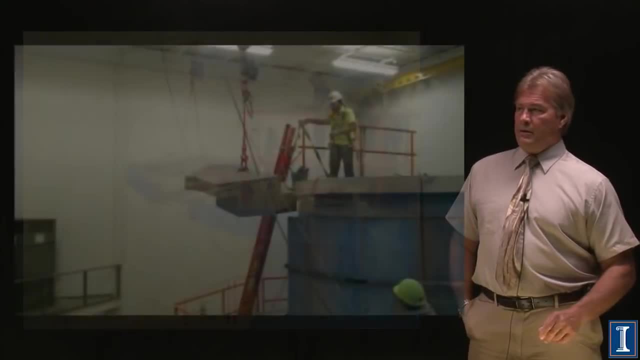 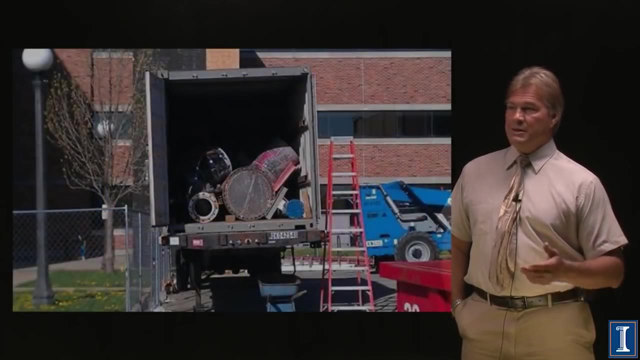 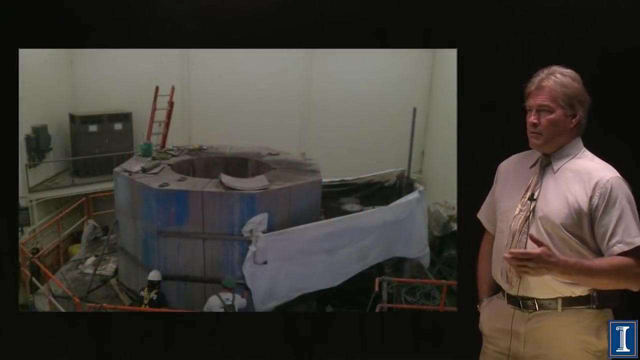 dismantle this. Well, you saw it off And you cart piece by piece away, And when you do this, it eventually ends up in a truck And the truck will take it to a low-level waste repository. When you get down a bit further and the concrete's very thick, 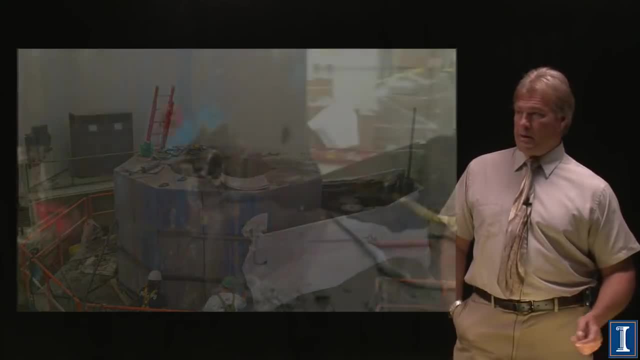 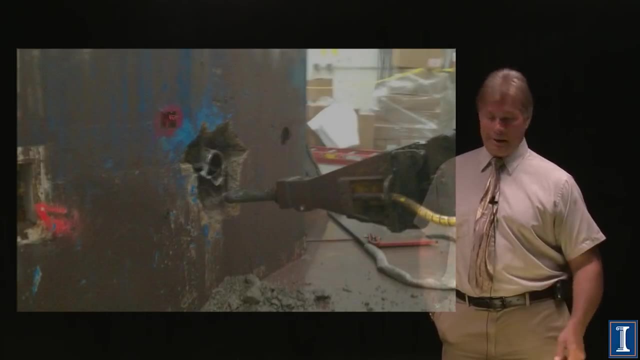 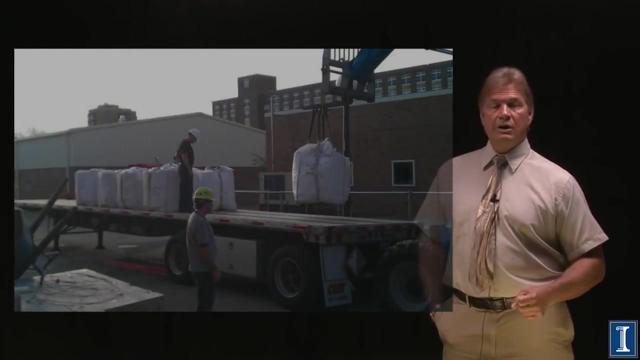 then you have to maybe take it apart in in the form of rubble At least, drilling out certain beam ports which you can take away and encase, And this stuff eventually also all ends up bundled and put on a truck and taken away and buried.